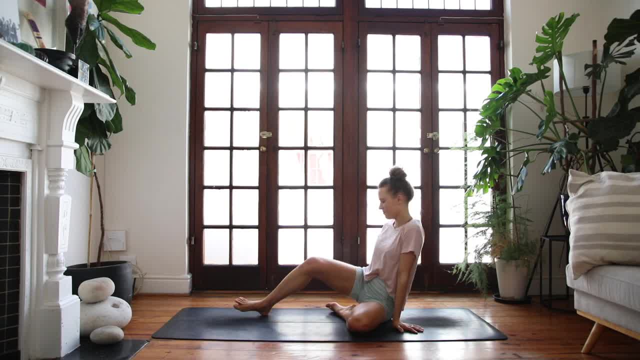 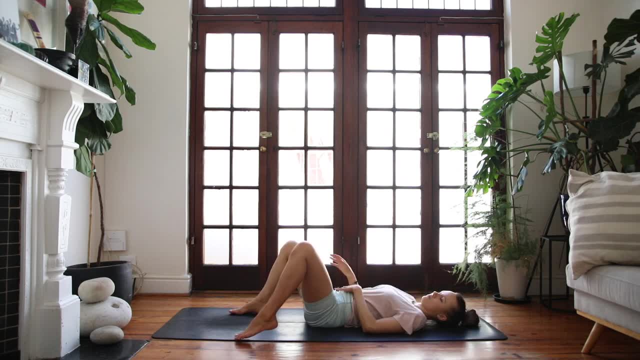 All you need is yourself and a yoga mat or a carpet So when you're ready, you can go ahead and start lying down on your back in constructive position of rest. So you can bring your feet out to the edges of the mat and draw your knees into each other and place your hands to your 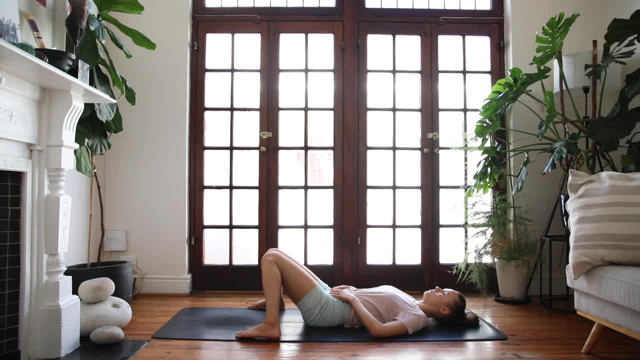 lower belly and try to relax the body completely, softening through your shoulders, your jaw, your face and your neck. I'm just inviting in a sense of groundedness, as you connect your breath, So closing the eyes. if you feel comfortable, We'll start. 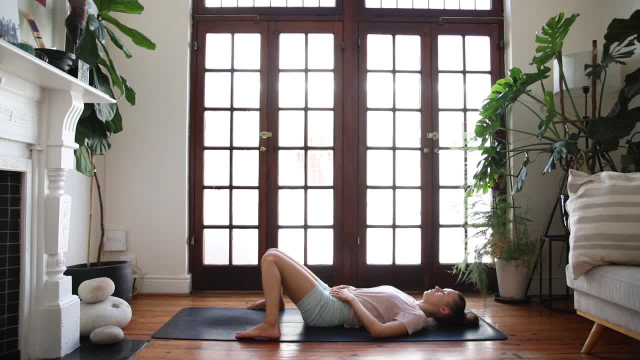 to deepen the breath, directing the breath all the way into your abdomen, your belly, Nice, full inhales, feeling the expansion as you breathe in and a gentle contraction as you breathe out, deflating completely. I'm just taking a few more rounds, just like this. 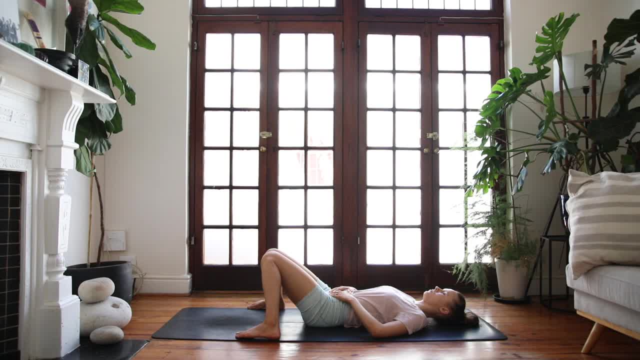 Just induce theia-anya to move and relax. once the offset of the bag is smelling into your mind's system, We're gonna celle into aih voix On your next breath in. find a wind removing pose. pull the right knee into your chest. 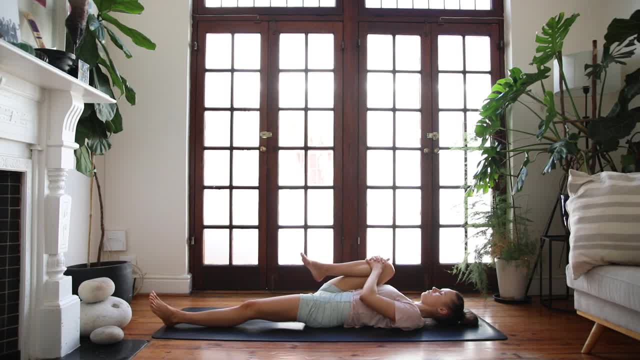 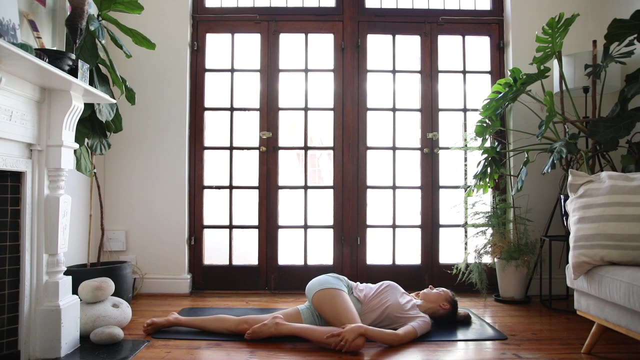 and interlace your hands around the right shin, Hugging that right knee in towards the heart space and give it a nice little squeeze here and then take that knee over to the left side in a gentle spinal twist. so this doesn't need to be a super deep twist, we're just trying to create a bit of. 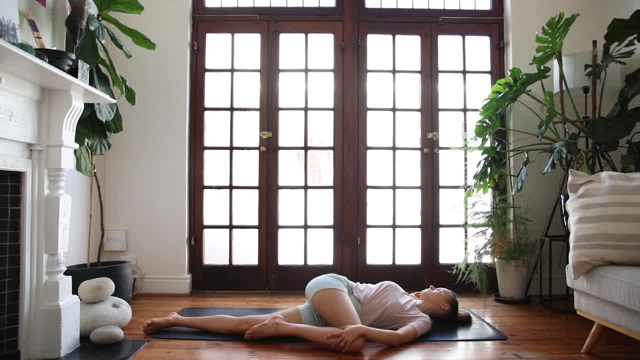 space here across the trunk, the spine, the lower back- not the right shoulder- as close to the floor as feels comfortable, and then breathe fully here into the right ribcage, finding a sense of spaciousness and really trying to keep the rest of the body as relaxed and as rooted as you can. 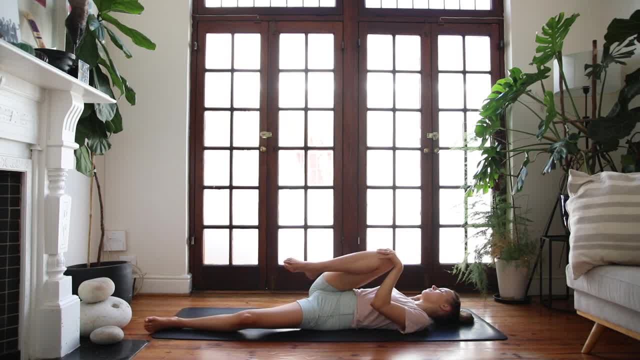 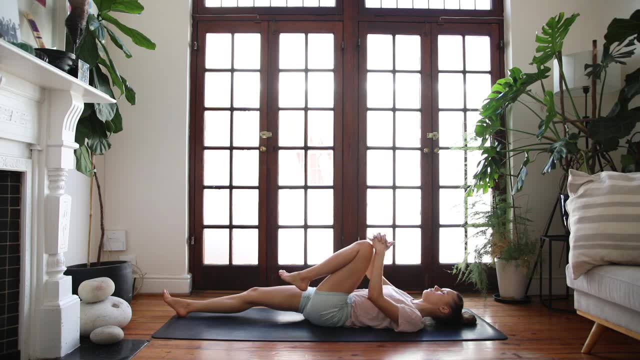 inhale. draw that knee back into the chest. exhale, send it forwards. let's change our legs. draw the left knee to your heart, hug that thigh in towards the heart space. give it a nice little squeeze here and then the right side and exhale. send that leg over to the right side to find your twist: melt the left. 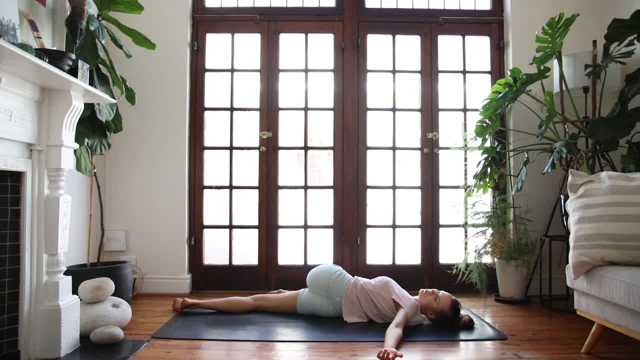 shoulder to the floor and take a couple of slow, deep breaths here, opening up a little bit more, allowing the body to feel a little bit more loose, a little bit more relaxed. with each breath out, start drawing your left knee back into your heart space and then find happy baby pose knees to your 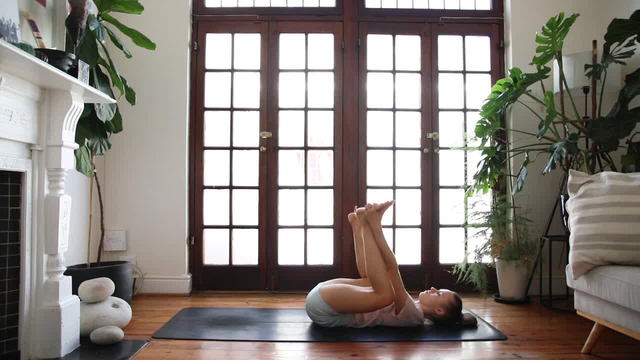 armpits, hands around the edges of your feet or around the thighs, whatever feels comfortable here. try to flatten your spine a little bit more and then take a couple of slow, deep breaths here, opening up a little bit more, as much as you can, to the floor. so try to really ground your lower back here. 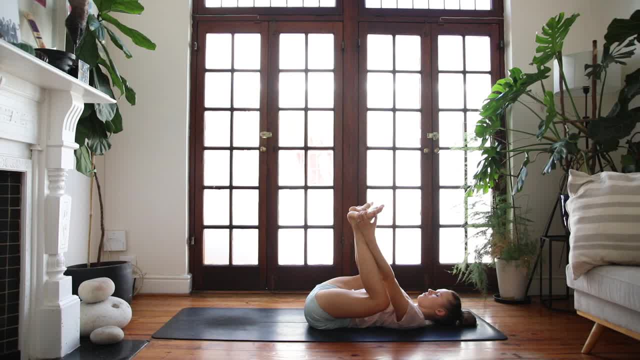 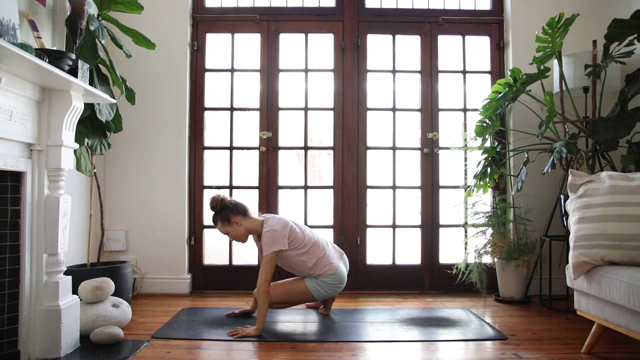 if your hands are around, your ankles begin to kick into your hands a little bit, creating a bit of compression here through the hips. okay, lovely, start to pull your knees into your chest and we'll begin to rock backwards and forwards on the spine. we'll meet in a tabletop position when you're. 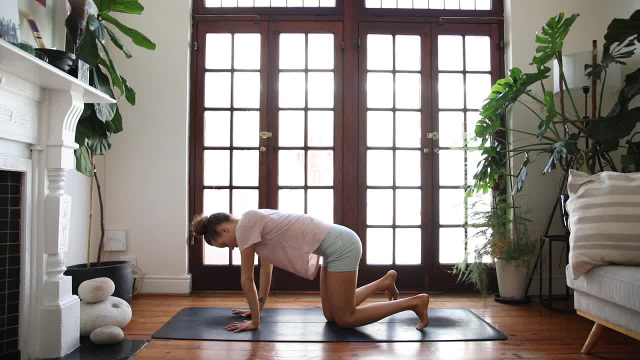 ready, coming onto your hands and your knees. bring your shoulders over your wrists and your hips over your knees. spread the fingers wide and inhale. arch the spine. find your cow pose. exhale round and contract the spine. tuck your chin nice and slowly breathe and arch through the spine. tilt the sit bones to. 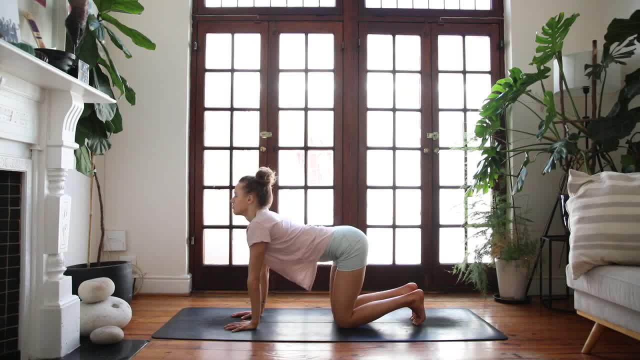 the sky. exhale round through your spine, curl your hips and bring your shoulders over your knees and style the tailbone to the floor. inhale, lift the chest, draw the shoulders down and back and exhale slowly. contract as you round through the upper back. beautiful, find a neutral spine and 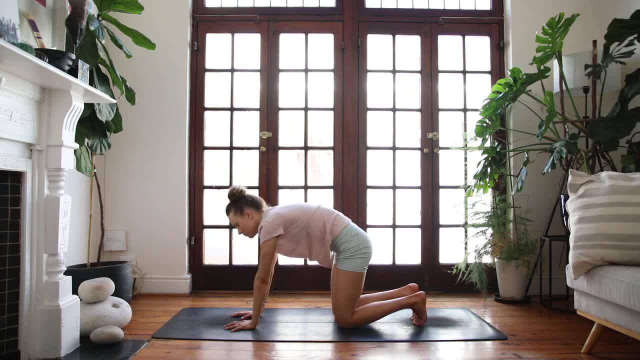 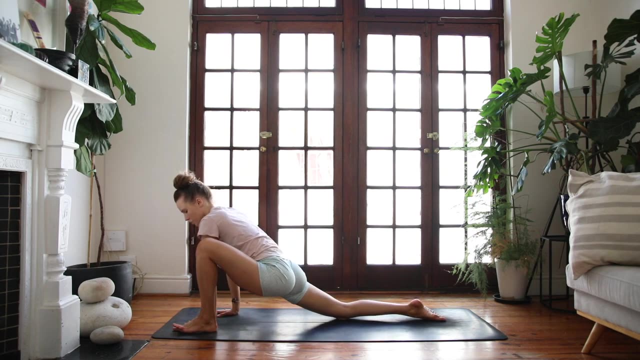 thenog 2010. beautiful. find a neutral spine and then step the left foot forwards to find lizard pose, keeping that right knee to the floor. ground your palms into the earth and start to pull the hips forwards and down. lift your chest forwards and up and we'll take a couple of deep breaths here, breathing into our 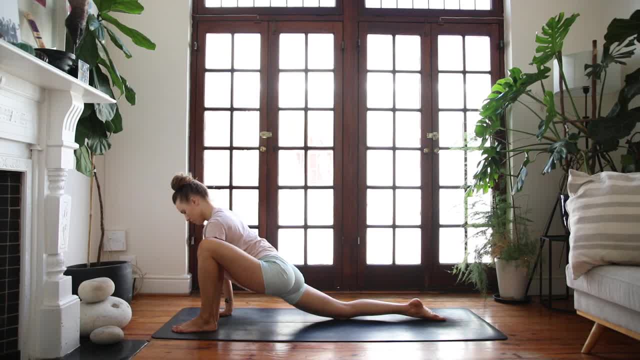 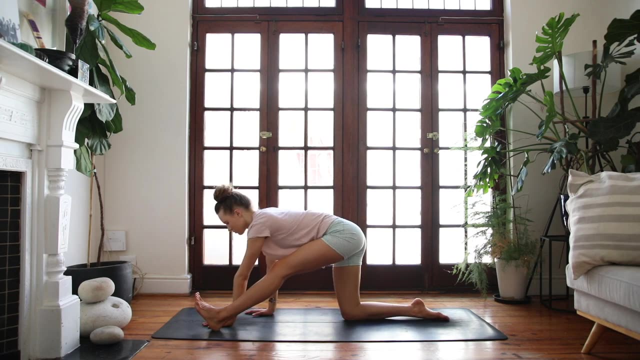 hip flexor on the end of your exhale. start to straighten out through your left leg. we'll find half splits. pose hands on either side of your left leg, flex through the left foot, toes pointing towards you, and breathe into your hamstring as we find a bit of space here. 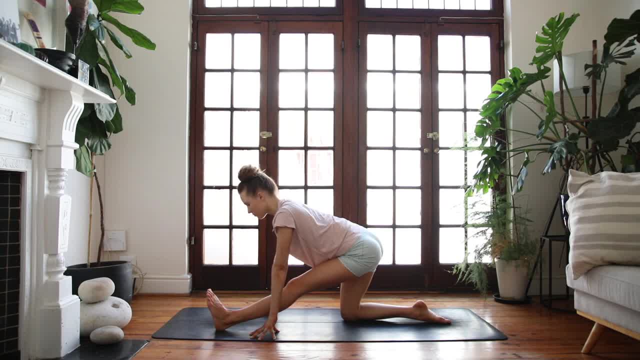 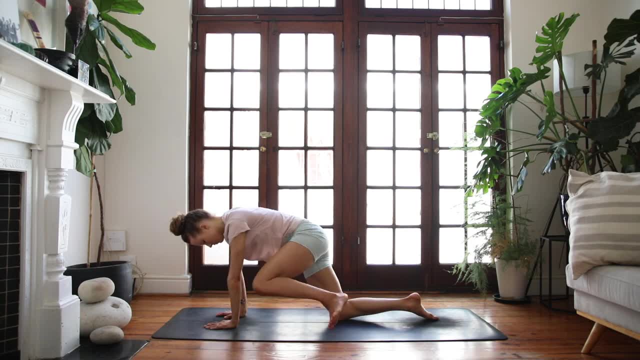 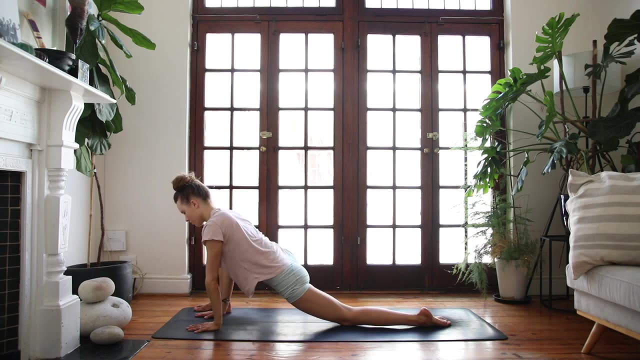 you start walking yourself forwards back to a lunge, exhale, left knee lowers, back to the floor. let's change sides. step the right foot forwards outside of your right hand and pull the hips forwards and down and take a couple of deep breaths here as you get a nice full stretch through your psoas and through. 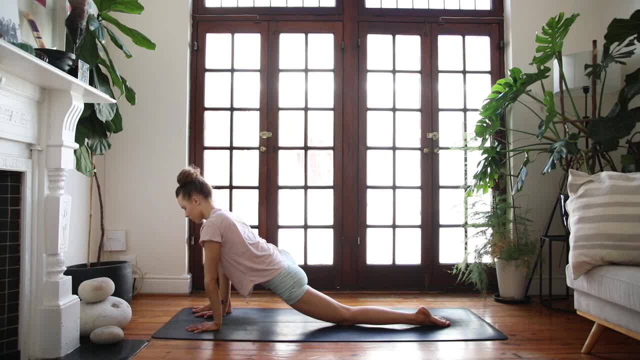 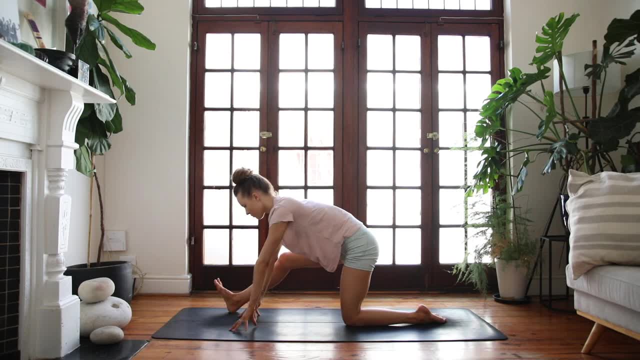 the hip flexors and then take a couple of deep breaths here as you get a nice full stretch through your psoas and through your day. we'll find a neutral spine, our BIGGest dead body. push up, welcome back into neutral. we'll put up that foot, as we have no 285. 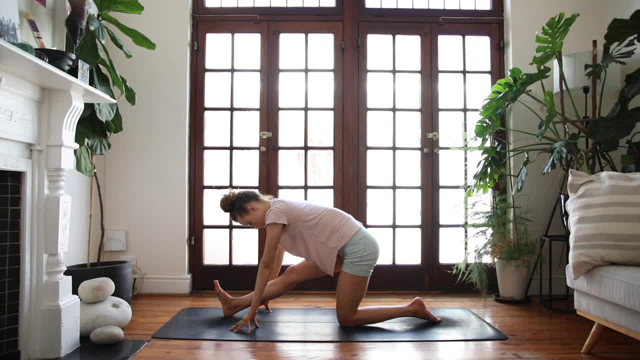 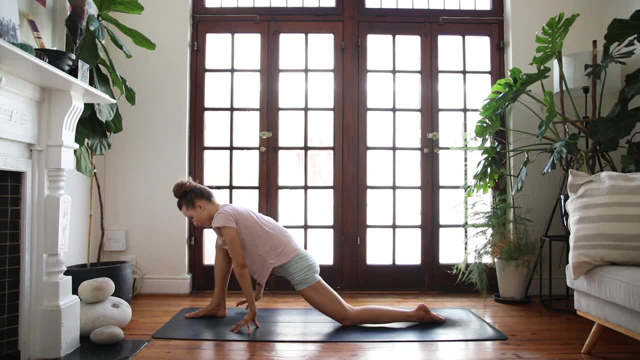 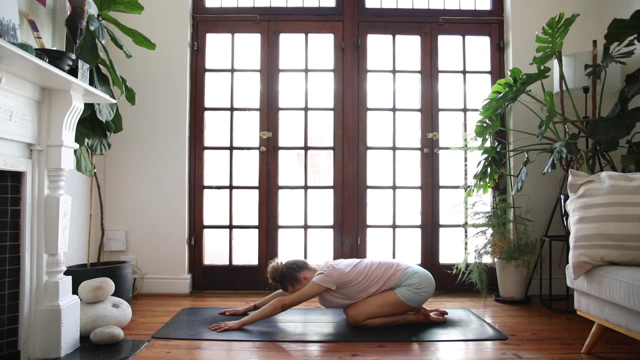 all low and then ground your palms into the floor. glide the right knee behind you. sit back into Balasana child's pose. you can wrap your hands around your heels. soften the forehead to the mat. we'll take five deep breaths here into our spine, so try to relax the body completely soft through the shoulders. 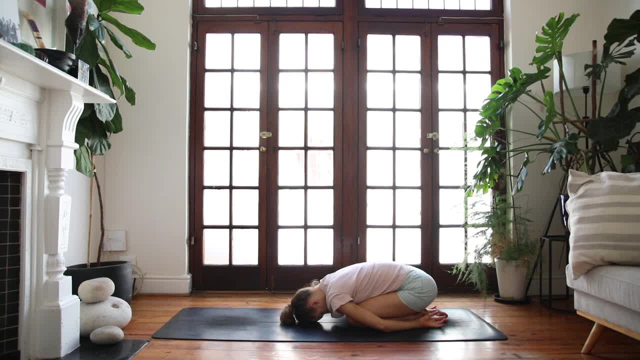 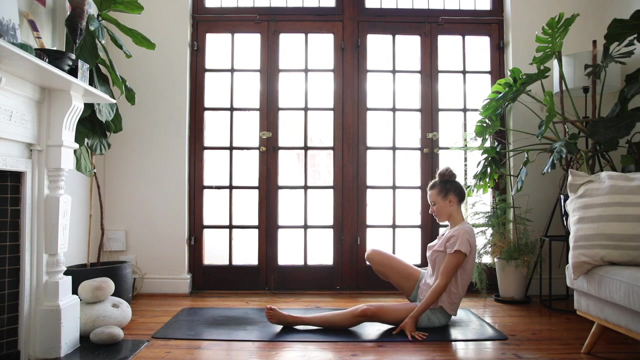 the jaw, the neck and feel a sense of spaciousness across the upper back, the middle of the back and the lower back. on your next breath, in gently lift your gaze and come into a kneeling position and then slide your legs over to the right side and we'll find a very loose 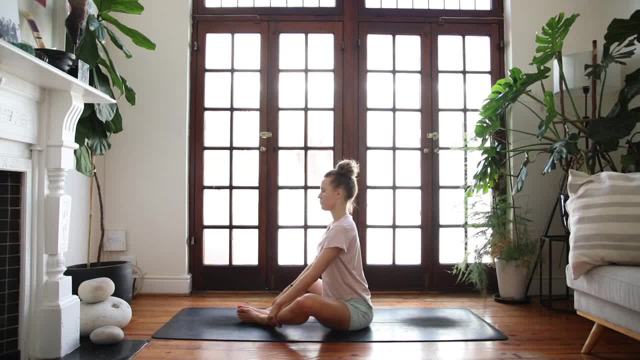 butterfly pose here so you can draw the soles of your feet together and then find a bit of length through your spine, exhale, fold forwards, maybe drawing your chest closer to your chest, and then bring your arms back to the floor, your feet- if this isn't comfortable and you're feeling really tight through your 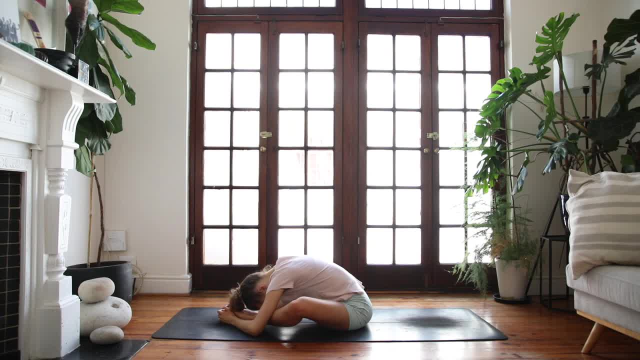 hips. just keep a bit of a longer spine. we're opening up here through our hips, our thighs and groin muscles as well as the lower back. but if anything is feeling a little bit too tight or tense in the body, just back off a little bit. sometimes deeper isn't always better at all. 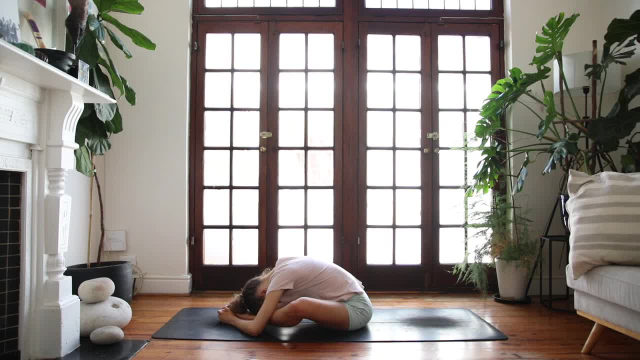 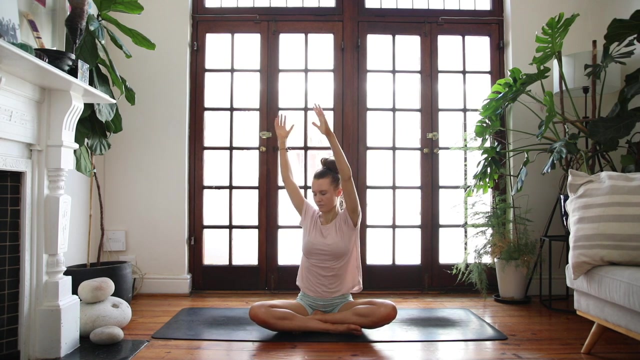 take three more rounds of breath: inhale, lift your gaze and lift your chest and come into our final position, a cross-legged seat placing the right foot in front of the left foot. inhale, reach the arms up, exhale. Exhale. twist to your right side, left hand to right thigh. 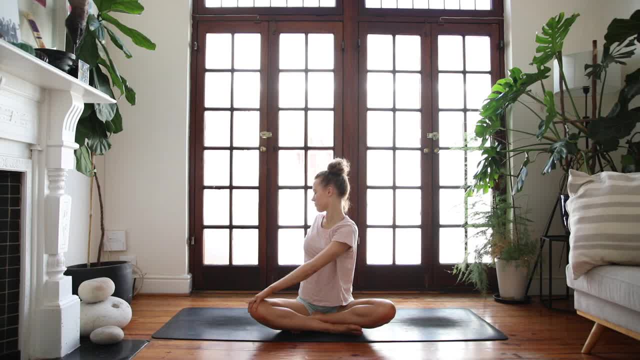 Stay long through your spine, face relaxed, And slowly unwind, coming back to the middle And exhale over to the other side. find your twist: Right hand to left knee, lengthening up through your twist, Slowly unwind, bring yourself back to the middle.